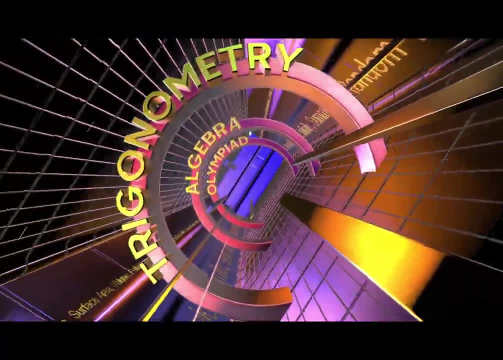 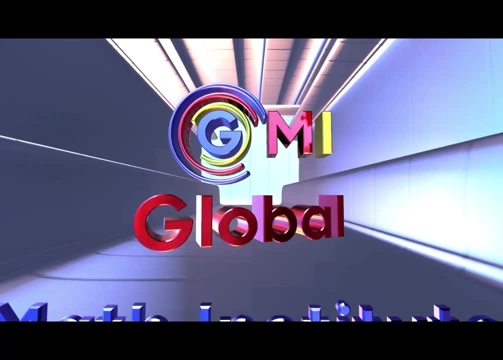 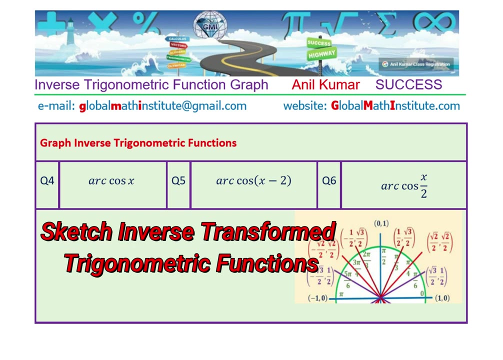 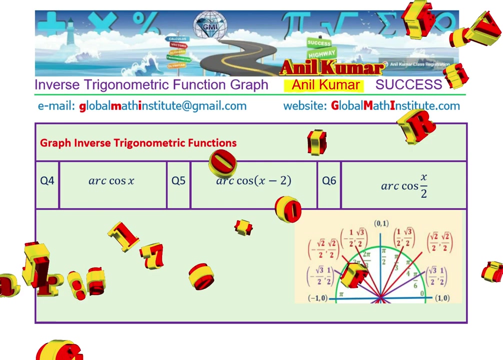 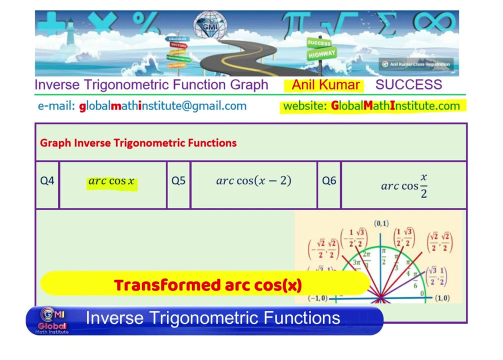 I am Andil Kumar. Welcome to my YouTube channel and the website Global Math Institute. In this video we are going to discuss arc, cosine, sine, inverse x and also graph when it is transformed right, So you can see the transformations. also. We are considering mainly horizontal transformations in this particular video. 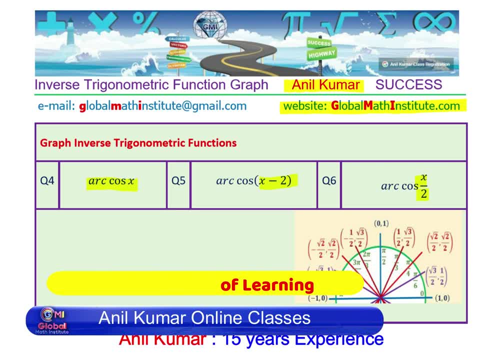 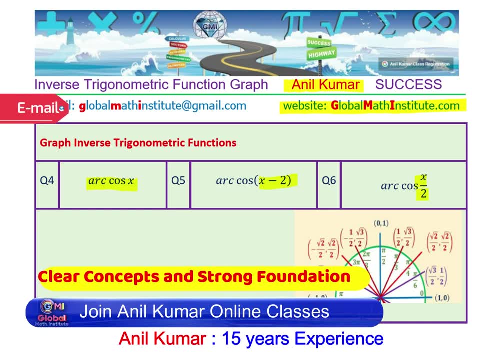 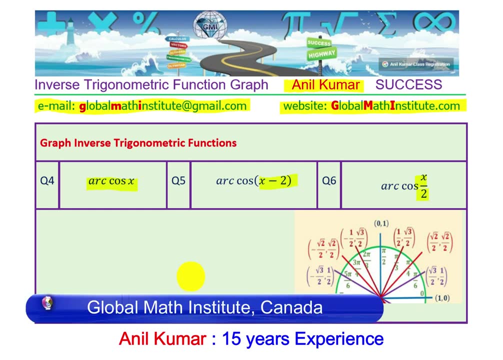 In the playlist you'll have wide variety of sketching graphs for trigonometric inverse functions. Well, in case you want to learn from me, feel free to send an email on globalmathinstitute at gmailcom. Our students are right there on the top. We can be part of your success story. 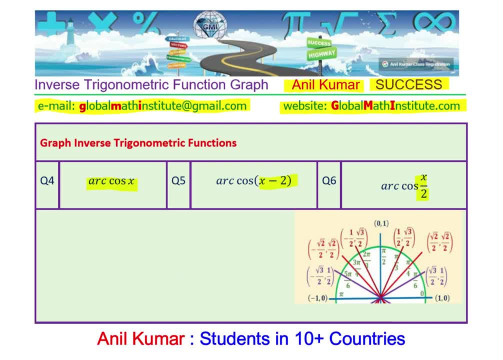 Now let's look into cosine function first, and then we'll get into the details. So I'm first sketching a sinusoidal wave, right? So that's my sinusoidal waves. Now, when we say cosine, it starts with the maximum. So let this be the starting point and then let this be the y-axis, x-axis. 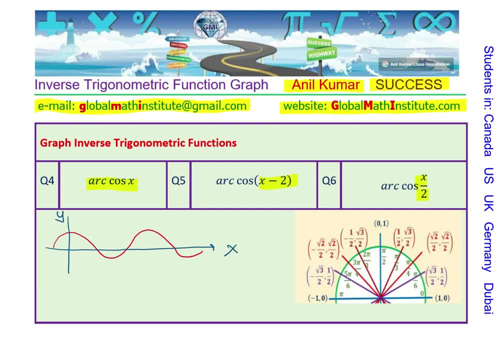 So this is x and this is y. for us, The cosine wave starts with the maximum, So 1 at 0 and minus 1, so it's not to the scale. at And at 2 pi we again have 1.. So that is the cosine wave. 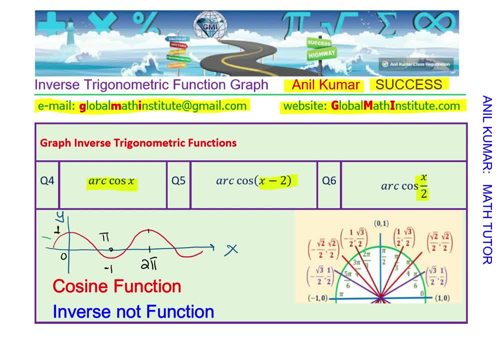 If I draw a horizontal line, you know it is going to cross at more than one point And therefore inverse of cosine function is not a function. right To make inverse a function, we have to do a restriction on the domain of cosine function. 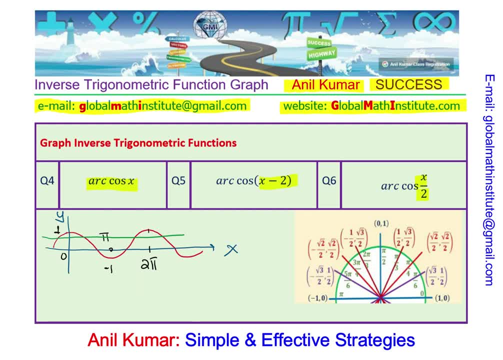 So the restriction done is we only consider from 0 to pi. So this half graph of cosine, that is the restricted domain. So now our domain for the cosine function has been restricted from 0 to pi. Well, those of you who are working in degrees can write 180 degrees. 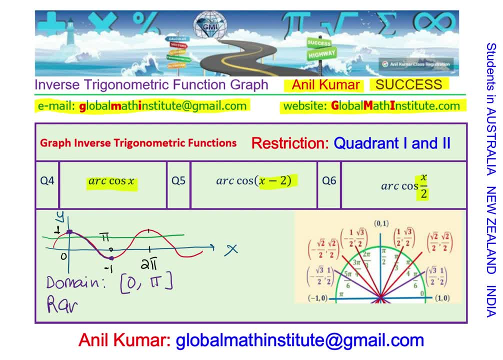 Now you can see, in this domain range is from minus 1 to 1, right, So our full range is there, So all the values which cosine can take, for that we can have an angle right. But we'll work only in the domain of 0 to pi. 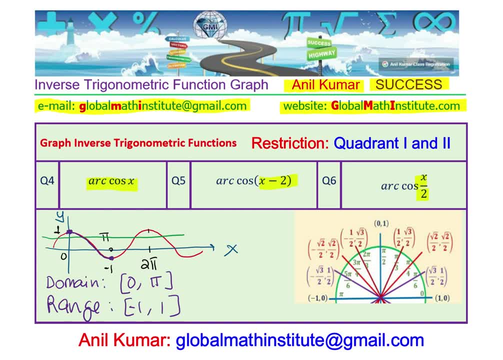 So whenever you have questions where you have to evaluate something related to cos inverse, always look into only the domain which is from 0 to pi. Does it make sense? Means in quadrant 1 and in quadrant 2,. as you know, in quadrant 1, all are positive right. 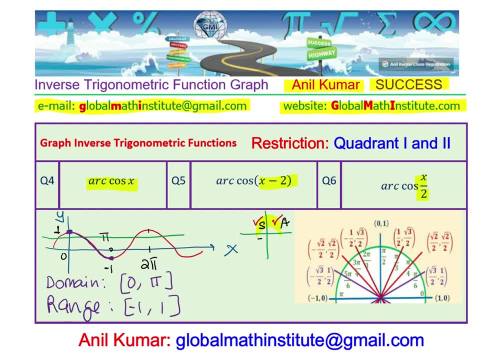 But in quadrant 2, sine is positive, not cosine, right? So that is the cost rule for you. So now we understand that we have restricted the domain of cosine function to ensure that its inverse is a function right Now, if you take the inverse, then the domain and range will swap correct. 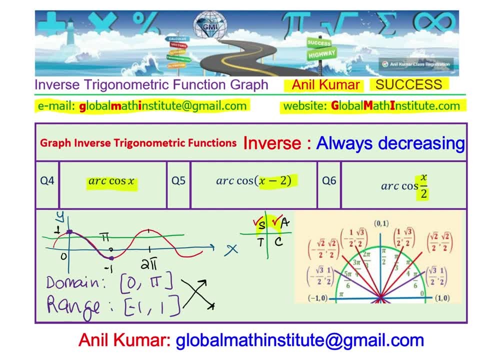 So for inverse, as we know, let me write down: This is the basic concept, So the domain for the inverse. so we'll write: cos, inverse x will now be from minus 1 to 1, and the range will be from 0 to pi makes sense. 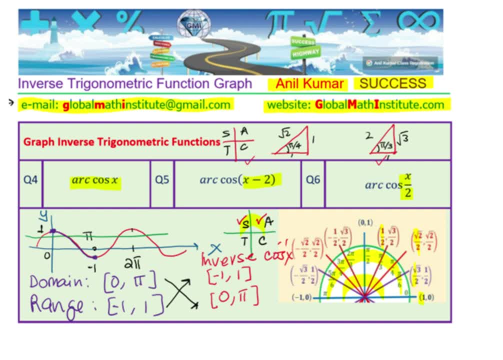 Correct. So with that in mind, we are going to sketch the graph of inverse cosine function. Perfect. So to do question number 5 and 6, we'll do the transformation of that particular graph. Now, this is from 4,, 5, and 6,, 1,, 2, and 3.. 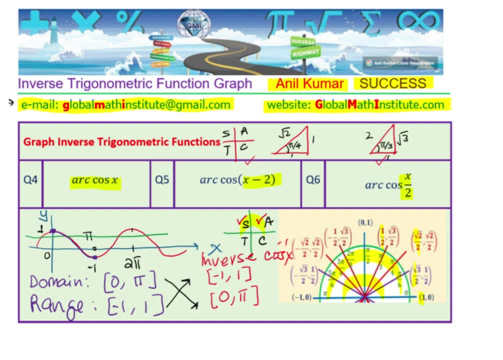 We had a similar discussion on sine functions with different types of transformations. So the idea is you learn all about transformations with trigonometric inverse functions with six examples, three of them, of each primary trigonometric ratio. So I hope it is making sense. 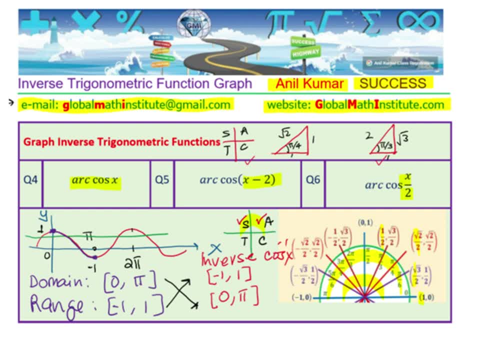 Now also, you will notice that. So you will notice that I only considered half of the unit circle Now. half of the unit circle because, as you can see, we are working only in the domain from 0 to pi for cosine function. 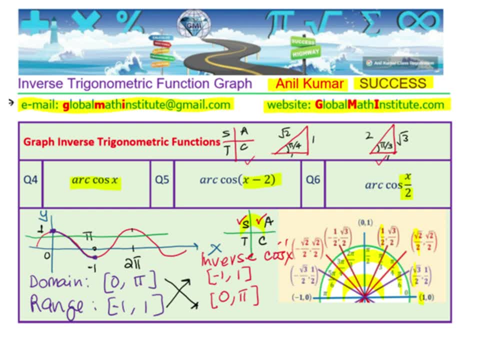 So all the values required are provided here. As you know, x values represent the cosine values for the different angles given inside the unit circle. Perfect, So that becomes your reference frame. Many stars. So if students are used to using unit circle, you can use that. 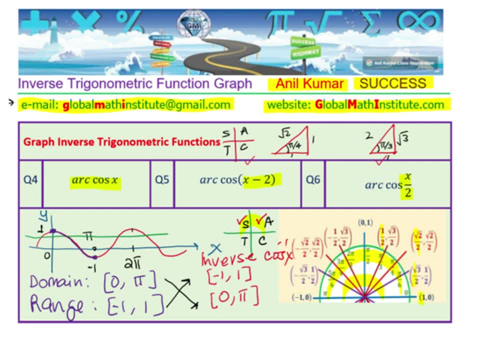 Most of you, which are my students, definitely use special triangles, So I'm making a special triangle here also. So we use these two special triangles most of the time and the cast rule correct. So we use these two things- cast rule to get the values, and the special triangles. 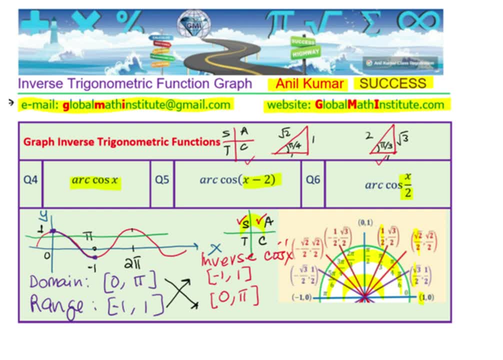 pi by 4.. For example, we'll have 1, 1 square root 2. And pi by 4.. Correct. And pi by 6,, pi by 3, we'll have 1,, 2 square root, 3, correct. 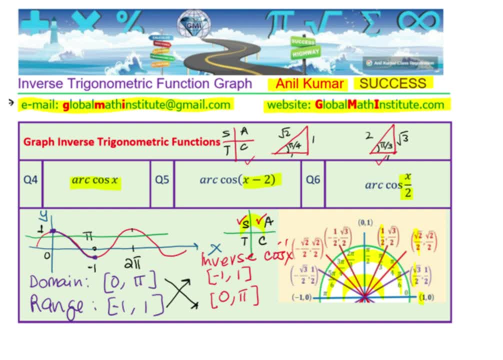 So you may use special triangles or the unit circle to get the values for sketching the graph. So rough sketch I will be providing, So I hope it is all making sense. It's very interesting to see how we are only using half of the unit circle so that we have 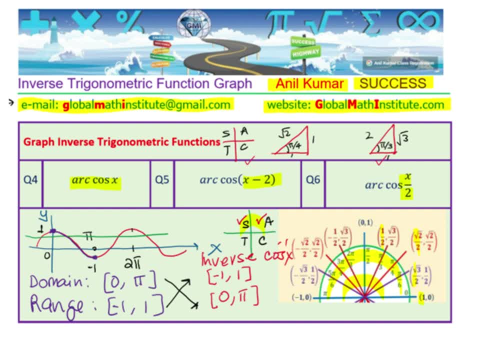 removed all the clutter, right? So everything which you need is there on the screen Makes sense, right? So I hope it is absolutely clear. If any doubts, feel free to send your questions on the email: globalmathinstitute at gmailcom. 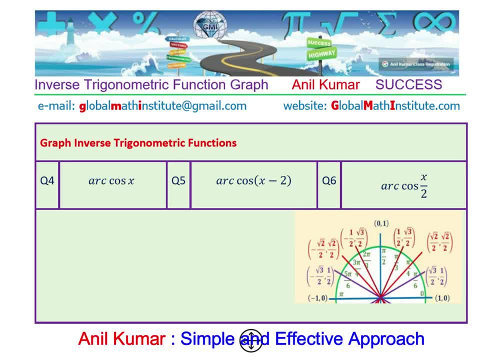 Now let's get back to sketching, right? So we just realized that for cosine function we have a domain which is from 0 to pi, right? So let's write on cos x here, Right? So for cos x, the coordinate points which we are interested in will be from 0.. 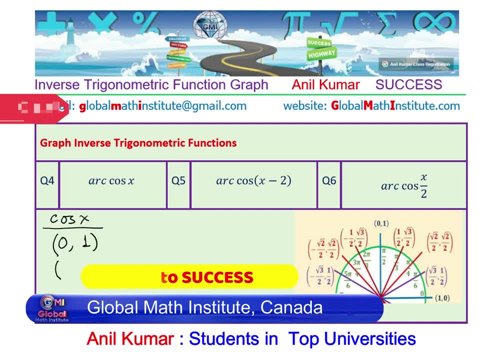 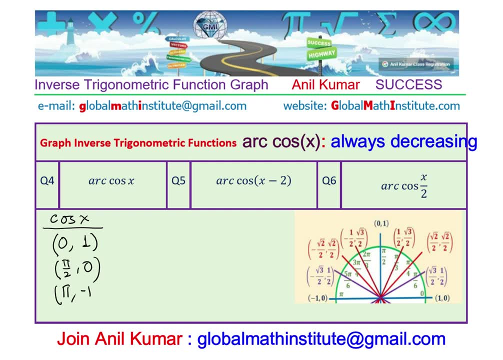 At 0, it is maximum value of 1. And then at pi by 2, we have a 0. And at pi we have minus 1, the minimum value. So it is always decreasing right. Correct 2 in. 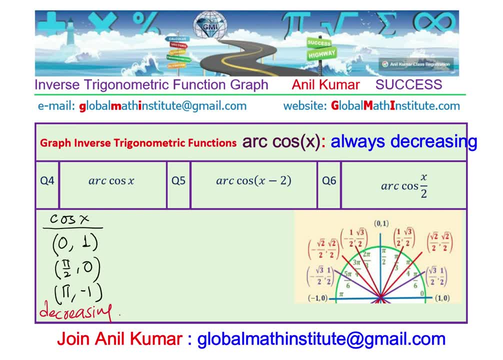 To sketch r cosine, let me write another yank right. What do we do? We swap x and y values, and therefore what we get here is value 1, 0, right, 0 pi by 2, and minus 1 pi correct. 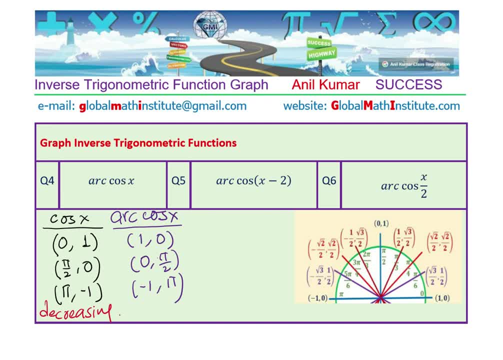 So you should also have in mind what is pi, right? So let's write down the value of pi. Approximately, it is equal to 3.5.. Correct. So pi by 2 is equal to 3.14, and pi by 2 is half of it, correct? 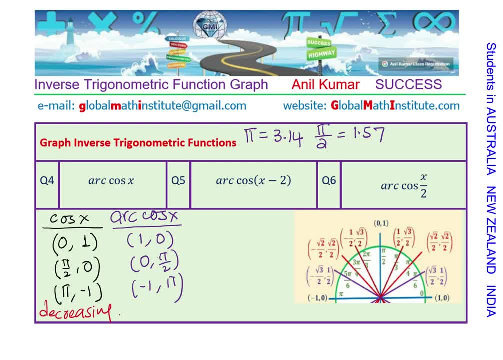 So 1.57.. So these are the approximate values of pi and pi by 2.. So you get an idea that pi is 3, more than 3 times 1.. So that gives you kind of a scale right. So I hope the concept is clear. 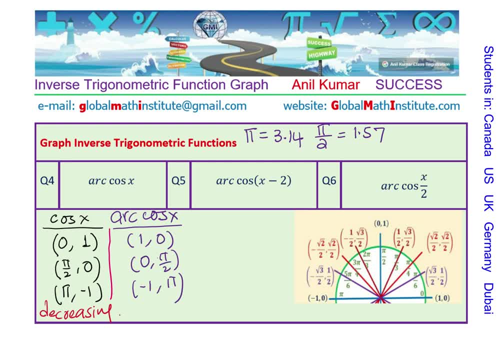 We have the points with us. We have the points for cos. We have the points for cos x and cosine, inverse x or arc x. Now let us try to sketch the graph for the same. So let me make a scale here. Most of it is on the upper half and therefore I'm drawing a line here. 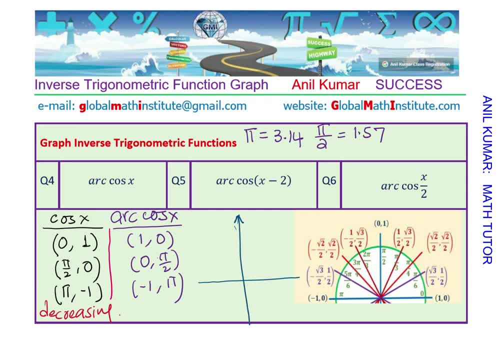 And there you go right. So that is my x and y axis. Let's put up a scale: 1,, 2, 3.. 1, 2, 3.. 1, 2, 3, correct. 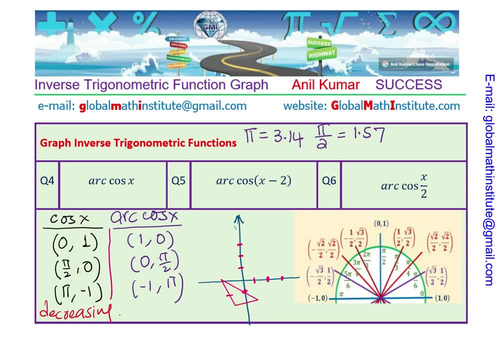 1, 2, 3.. Correct Right: 1, 2, 3,. correct minus 1.. Correct, So these are each units of 1, correct. Now, as you know, pi is 3.14, and pi by 2 is 1.57.. 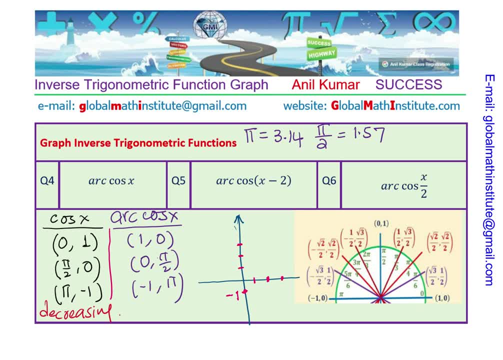 So at 1, we have a 0. So the first point for the cosine inverse will be right there, right, So we have taken the değ and the cosine, Okay, Okay, taken up this point, which is: at 1, we have 0.. Now, at 0, we have pi by 2.. Pi by 2 is: 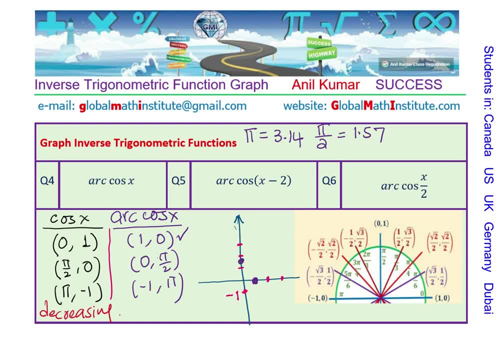 1.57, right. So that will be our second point. Is that clear? And at minus 1,, which is right there, we have pi, which is slightly more than 3, correct? You get the idea. So the 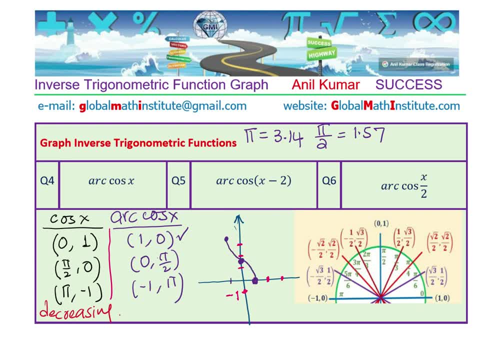 graph will be kind of like this: So that is a graph of cos inverse x, or r cos x. Is that clear to you? So this point right on the top is actually minus 1 pi, And that point here is 1, 0, the x-intercept in this case, right. So that is cos inverse x. I will also 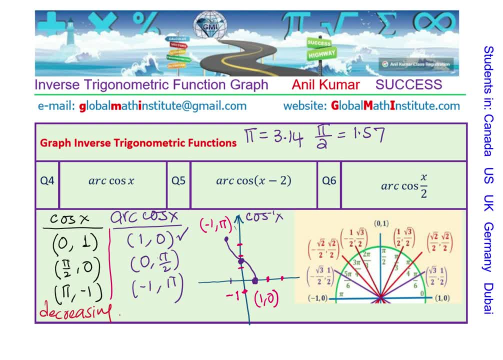 sketch on the same scale, The graph for cos x. So cos x was 1 here, right 1.. And at pi it was minus 1,, correct, And pi by 2, which is more than 1, it was kind of like this. You see that That is a. 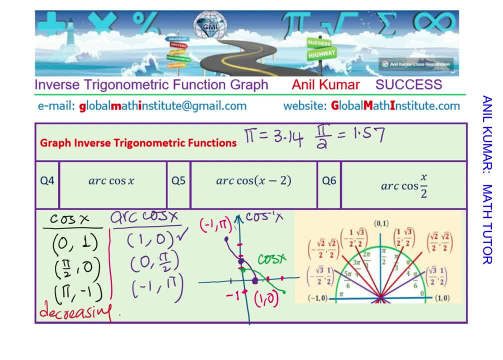 graph of cos x. So cos x graph, which was from 1 to minus 1 and from 0 to pi, has been reflected on the line which you know is y equal to x, to give you the inverse. Now you can very clearly see how we sketch the inverse of cosine functions, correct. 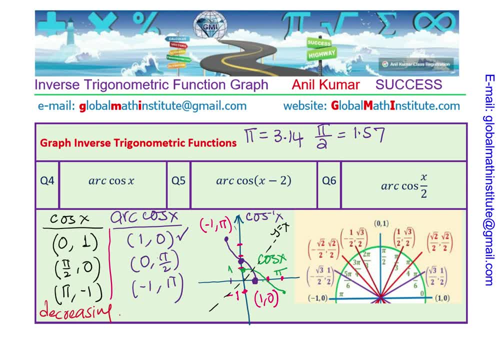 So the critical points to show those which are shown here: right, So pi by 2 is the y-intercept, 1 is the x-intercept and the maximum point is minus 1 pi. Right, So y is. 0,, et cetera, et cetera, And desktop amigos, than is the inverse of cosine functions correct? Now, if you see the centers of the strategic example numbers, which is divided by 2, right From Erich nephew. 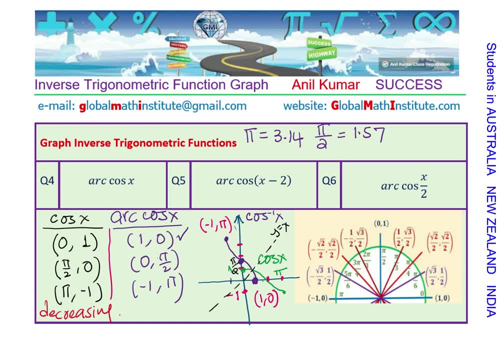 1, pi clear. So with that we have done question number 4, which is sketching r cos x. Now for getting more values you could have. so we use these values. at 0 we use 1 correct and at pi by 2 we use swap this value and pi. So in the unit circle only quadrant 1. 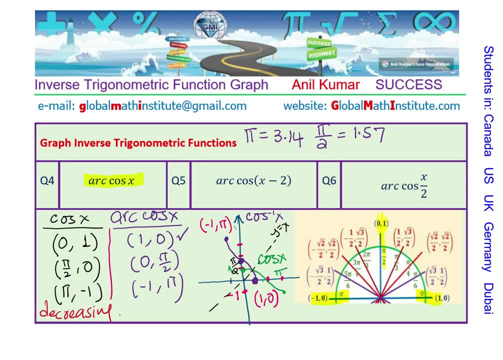 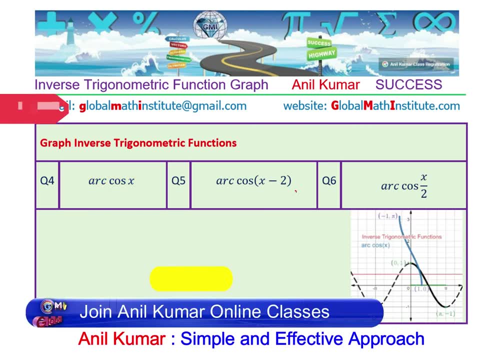 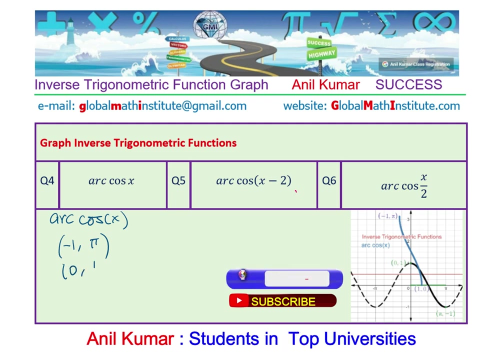 and 2 takes care of cosine inverse function. is that clear to you? Now let us do part b right. So let us rewrite the values r, cos, x, r. So at minus 1 we have the value of pi, then at 0 we have pi by 2, and at 1 we have 0, correct? 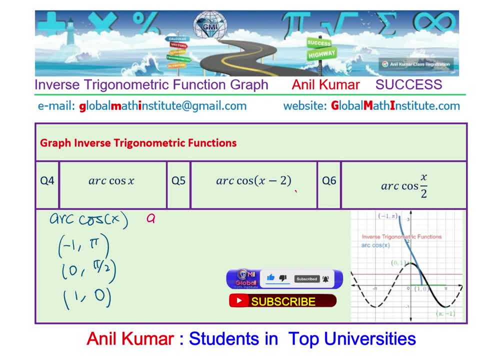 Now we need to sketch the graph of r cos x minus 2.. So what really happens? the coordinate points x, they move right. 2 units right. So translate: 2 units right, clear. So that means the x values will change right. 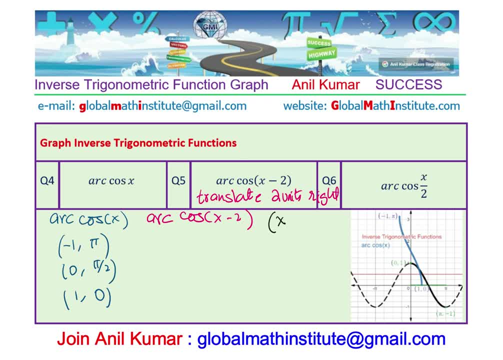 So the x values will now be plus 2, right, So x plus 2 and the y values will remain same. So let us write the new x values. Adding 2 to minus 1 will give me 1, pi will remain. 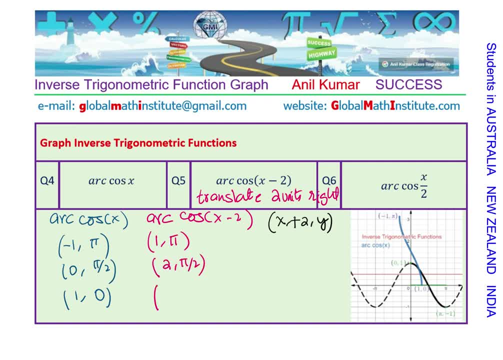 as such. then here will be 2 pi by 2, and then here it will be 3: 0.. So these are the new values. put them on the graph. I have already taken the graph of cos inverse x right. So. 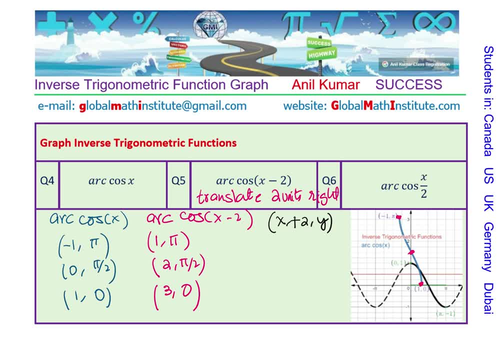 we are going to shift each and every point 2 units to the right. So the first one, which is minus 1, goes to 1, right, ok, So this is where it moves. The second one goes to 2, correct, So it moves here. The third one goes to 3, slightly less. 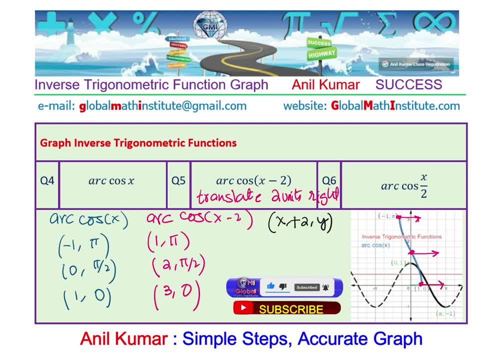 than pi. right, and connecting them, we have our graph. Is that clear? So that is how we are going to sketch the graph of cos inverse x minus 2.. Make sense, Easy, Perfect. So with that we have understood how do we take advantage of the cos inverse x and then sketch transform functions. At this point I 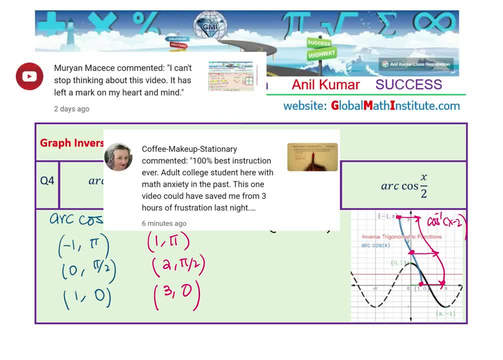 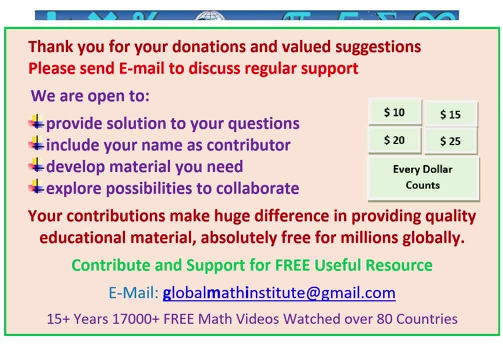 like to thank all my viewers and subscribers for watching my videos, posting excellent comments and suggestions. Some of you have been contributing. As you know, we provide absolutely free services. that too, since last 15 years, with more than 17,000 videos. The quality education. 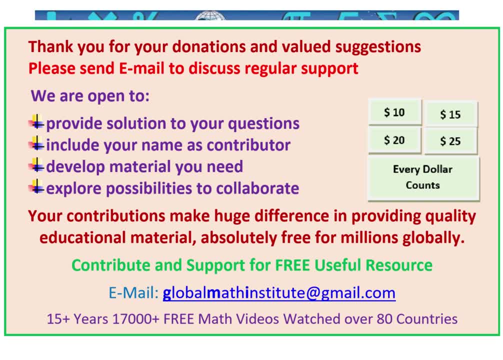 which we provide is very important. We provide absolutely free services. that too, since last 15 years, with more than 17,000 videos, The quality education which we provide is accessible to many students worldwide- more than 80 countries. Many do not have much privileges, as you have. 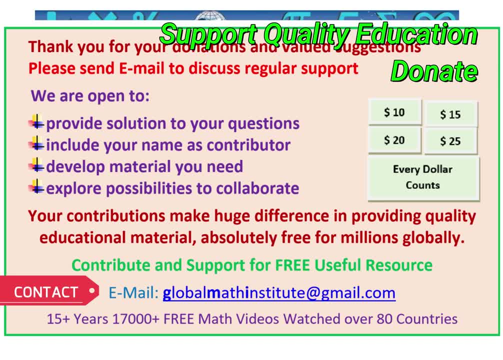 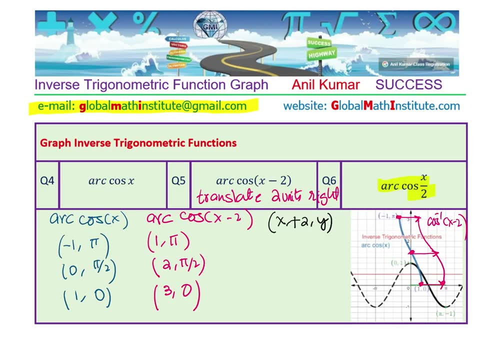 If you can donate and contribute help towards quality education, please do contact me on the email address given here. Perfect, And now we are going to take the last part of this question, which is again a horizontal transformation. I hope you can sketch it on your own. 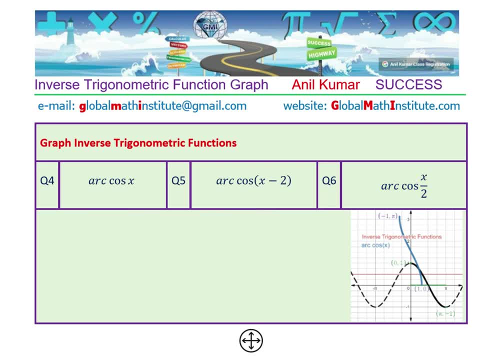 Some of you must have done it by now, right? So let us see how do we sketch arc cos x by 2.. First step: what is the transformation? Well, it is horizontally stretched by a factor of 2 right reciprocal of half, which is 2.. 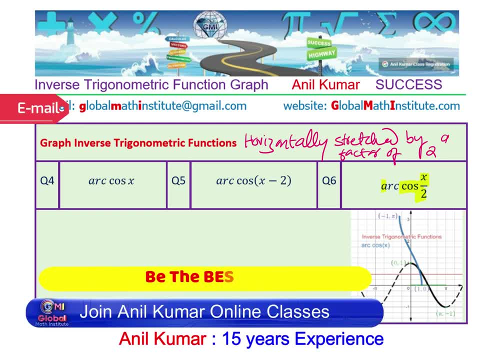 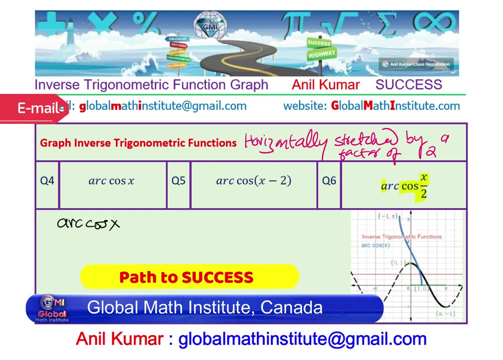 So we are looking for a wider graph, right? ok? So again, begin with r cos x. So let me write down the coordinate point for r cos x. this is going to be a process, correct, starting with minus 1 pi, correct? 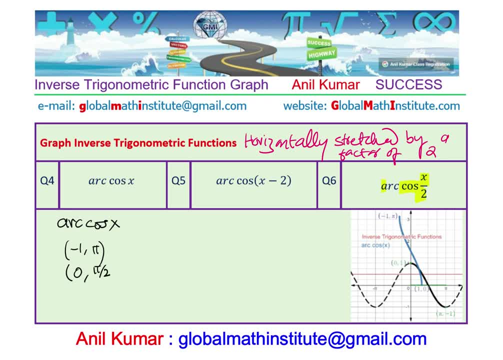 So the numbers and the radians, right. do you see? it becomes easy to do it. right? you get the idea. And then we will write down this time: arc cos x by 2.. So the x value will double up. so minus 1 becomes minus 2, the y value remains same. 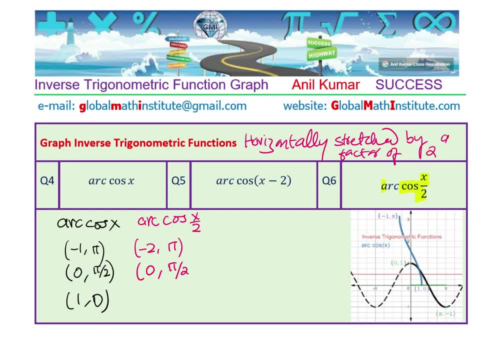 in this particular case, 0 will not change, And I mean the y-intercept. the 0 will become at 2, right, ok, great. So what you literally see is that the maximum moves one more unit towards the left y-intercept.